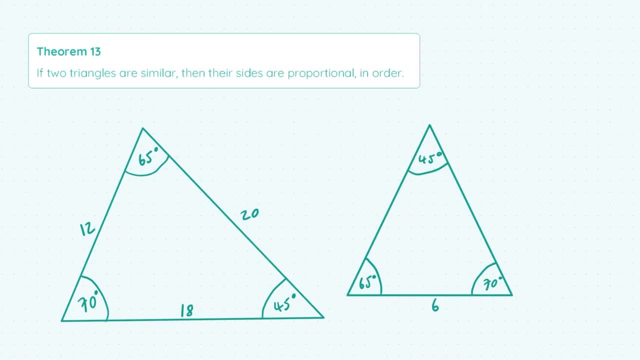 So with that out of the way now, let's just jump into an example. So, as you can see, we have two triangles here and they have the same angles, And note that the orientation here isn't the same. so our triangle here on the left is actually got 45 degrees in the bottom right corner. 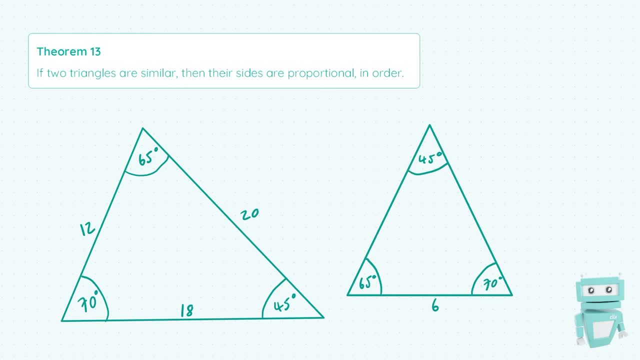 and our triangle on the right has 45 degrees at the top, but that makes no difference to what this theorem means, which is to do with the sides. So essentially, when we have two similar triangles, let's say we take the length of one side and increase it. 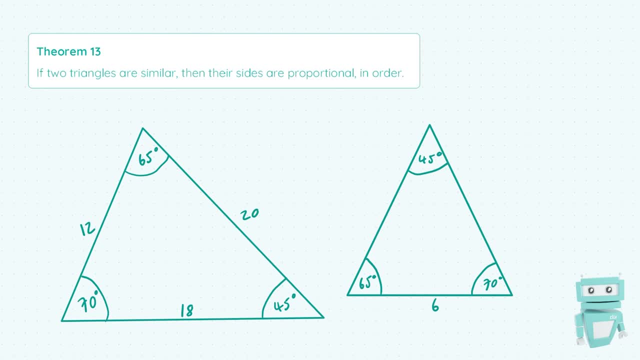 the other side lengths in the other similar triangle will increase or decrease proportionally to how we change the first side length. So in this case here you can see that in between 65 degrees and 70 degrees we have this side length 12,. 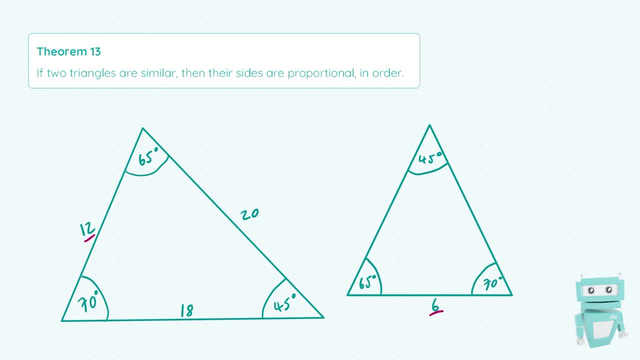 and this corresponds to the side length 6 in the second triangle, because this is positioned, once again, between 65 degrees and 70 degrees, And so all we can say is that the other side lengths will essentially change proportionately. So the fact that 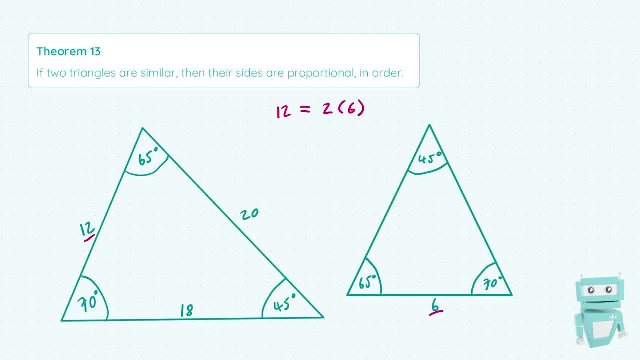 12 is equal to 2 times 6 means that the ratio here between our side lengths is going to be 2 is to 1.. So the fact that we have 12 on the left in the left triangle and 6 on the right